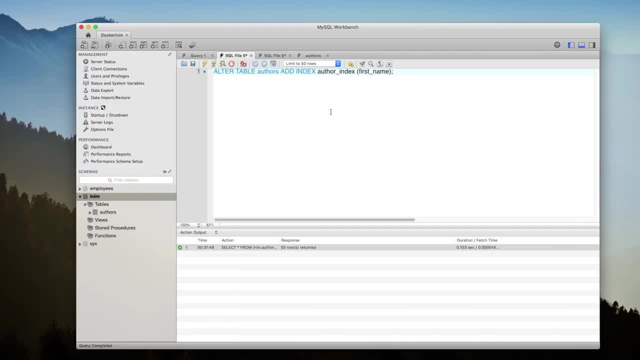 we can create indexes for multiple columns. Here I'm using just the alter table statement and I'm creating a new index by saying add index, the index name, which is the author index, and just one column, which is the first name column. Let me create this index, So you see. 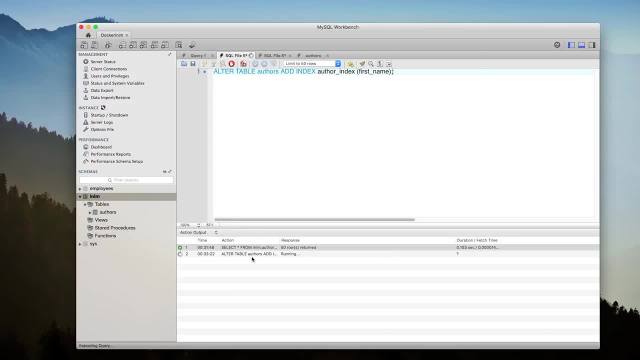 it's taking some time because when you create an index, MySQL has to take all the values from the first name column and store it in a separate location in a certain order, so that searching is easier and quicker. The index is done. Let's run the same query again. 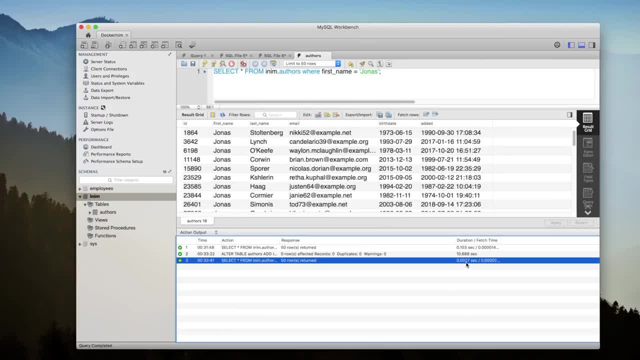 You see it was much faster. Notice that it took 0.0027 seconds, That is, 2.7 milliseconds. So the query went from 103 milliseconds for the same 50 rows to 2.7 milliseconds. Now that is fast. 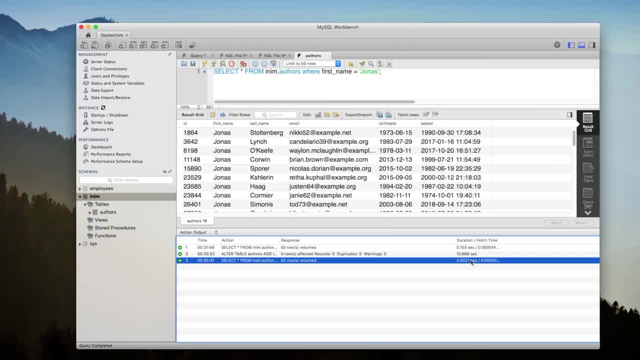 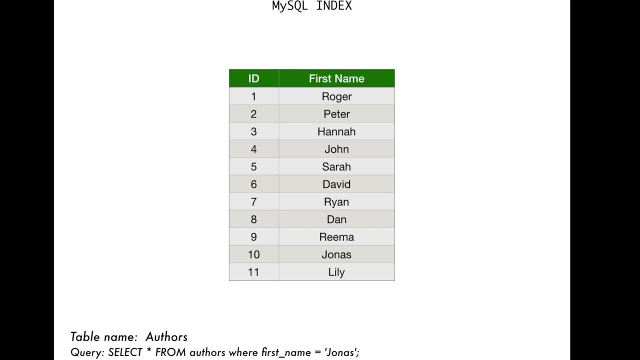 Now let's see how MySQL index works and how it worked with this example. Now here I'm showing the authors table without the other columns and just the first name column. to make it simple, I want us to think of database indexes the same way. 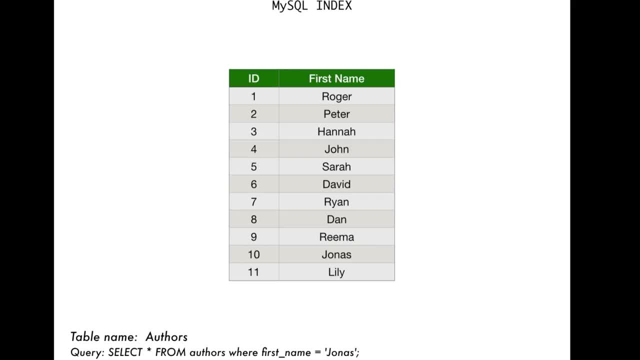 how the index in a book works. When you're searching for a certain word, there are two ways you can find it. You could either go through each and every page, or you can go to the index, find the word you're looking for and then go. 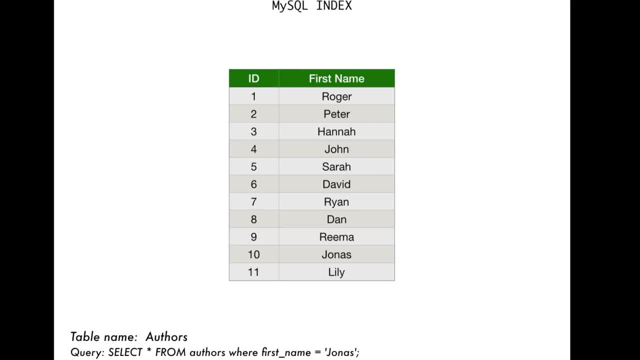 to the relevant pages. MySQL indexes work the exact same way. Now, when I'm searching for the word Jonas Now, without an index, MySQL would scan through each and every row till it finds the values Jonas. When it does, it will mark down the location. 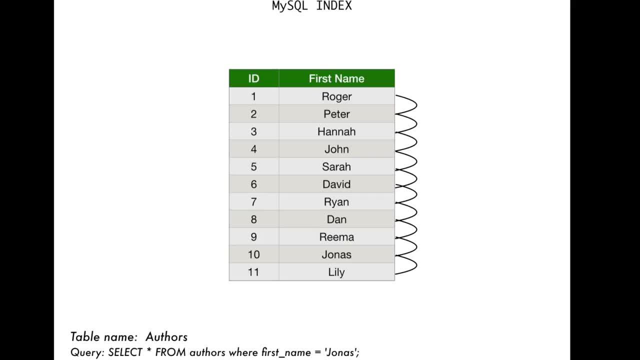 where it found the word Jonas, and then it will move to the next row till all the rows are scanned And once it's done it will go back to the locations where the value existed. it will pull out all the data and present to the user. This is why. 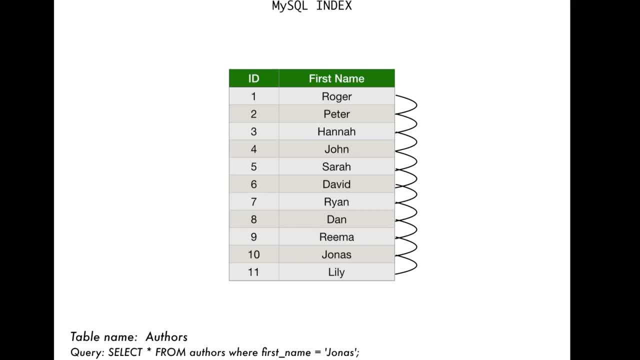 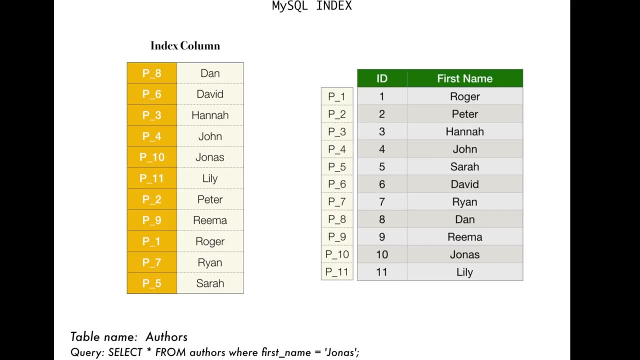 regular searches or regular filters are slow because MySQL has to go through each and every row. Now let's see what happens when we create an index. First notice that to the left of the author's table we have all the pointer locations. These are just locations. these are basically pointers which point to 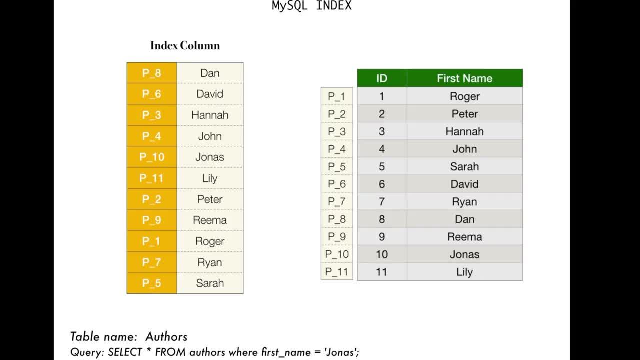 different locations. in the author's table To the left, we have the index column. Here what we notice is, when the index is created, MySQL takes all the data from the first name column and stores it in a separate location, and that's why it took. 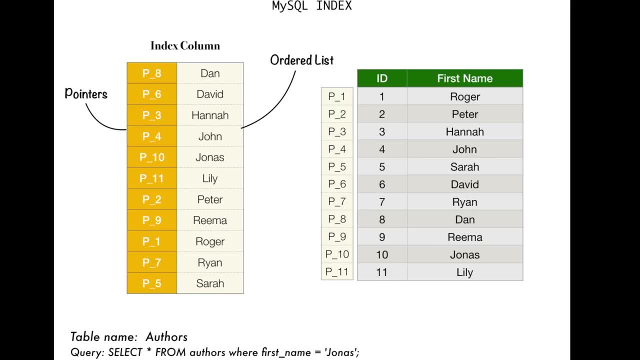 some time because it had to create separate storage for it. And you notice that it's set it up in an ordered list And it's also made a note of all the pointer locations. Now, this is basically how a B-tree structure works When we 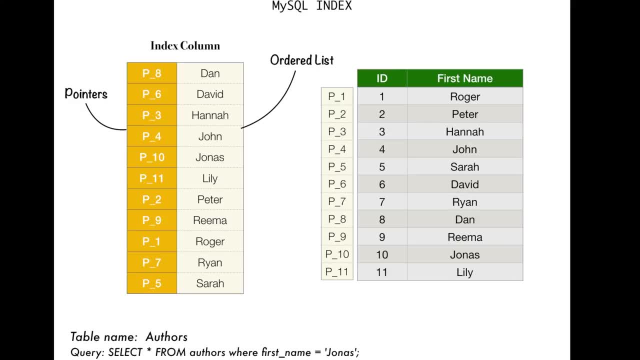 index, think of it as a B-tree structure. When we index, think of it as a B-tree structure. Now, this is basically how a B-tree structure works. When we index, think of it as a binary search. So when we search for Jonas, what MySQL does now on the index? 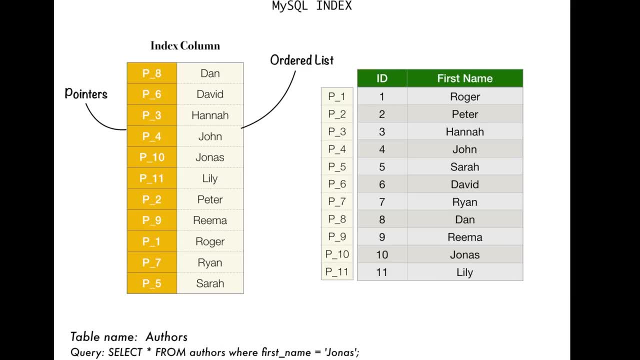 column is. since it's ordered, MySQL will know that each and every value, in terms of its byte value, will be greater than the next one, And so, when you're searching for the word Jonas, it will first look at the middle value of this column, which is Lily, and then it will check if the value of Jonas in byte is. 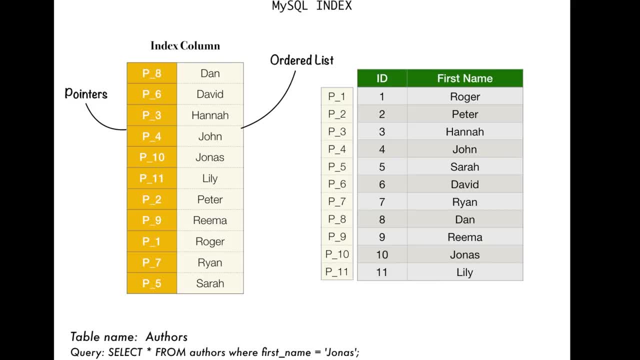 lesser or greater than Lily. If it is greater, it will look to the right of the column or, in this representation, bottom below Lily. If it was lesser, it would look above. Since the value of Jonas is lesser than Lily, it will look above Lily. The same procedure will continue. Next it will. 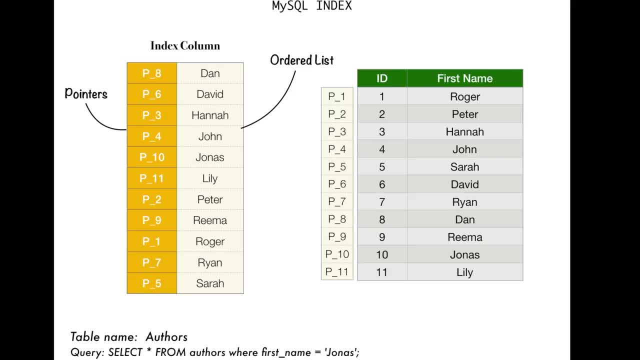 look for the middle value among the top row, which is Hannah, and then again it will check if it's greater or lesser. By this method of elimination, MySQL can find Jonas without having to look at the bottom row. So when we look at this, having to go through each and every row in the column. 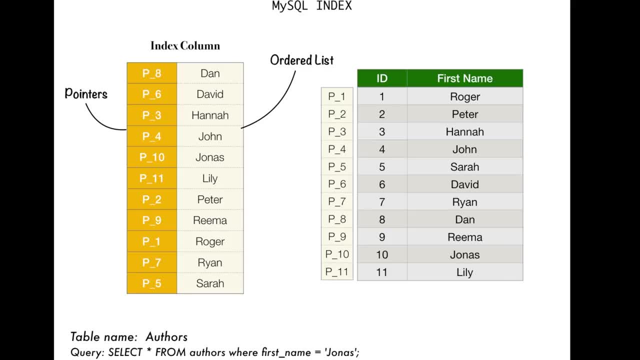 Once it finds a match, which is the value Jonas, it will check each and every row below it till it continues to find Jonas, And when the next word is not Jonas, it will realize that it's found all the values, which is equal to Jonas. 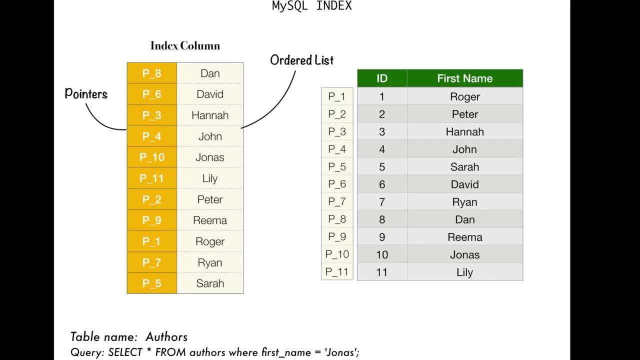 It will now take the corresponding pointer locations, which, in this example, is just p10.. It will go back to the original table, which is the author's table, pull out the data from the pointer location p10, and present it to the users.